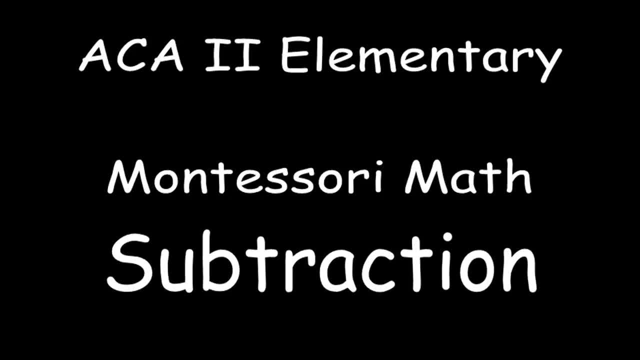 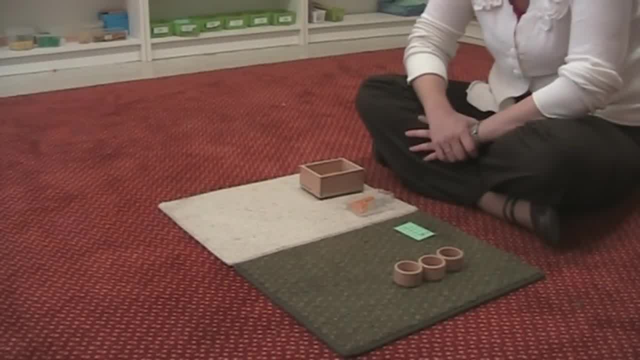 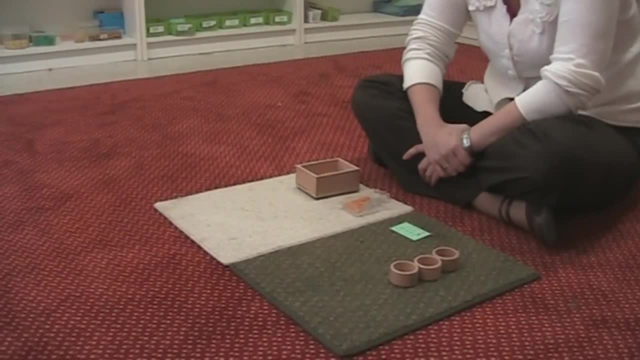 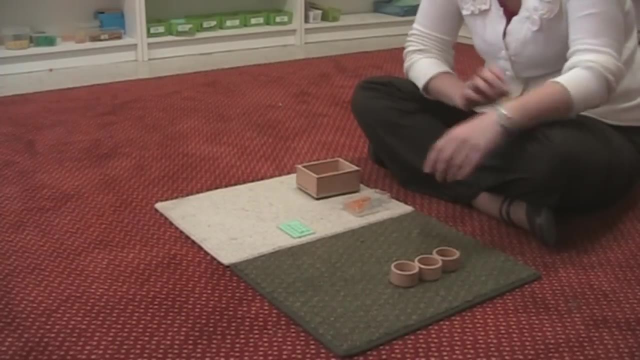 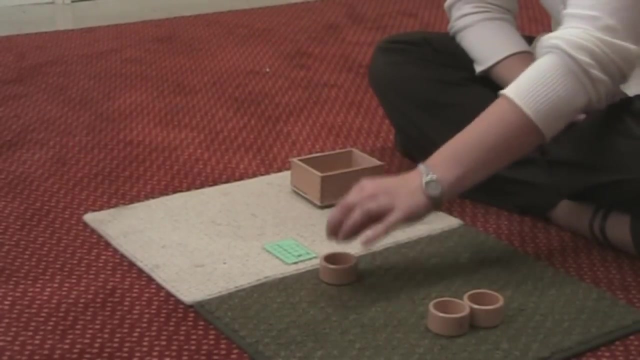 Okay, we're going to start with static subtraction using the golden beads. This is what the six and seven year olds would use to complete this job. We're going to start with seven minus six. In our first cup, we will count seven beads: One, two, three, four, five, six, seven. 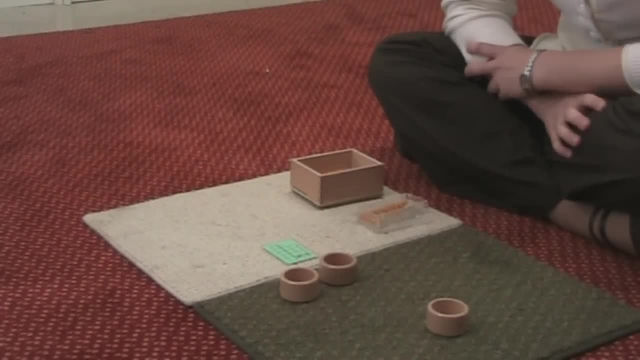 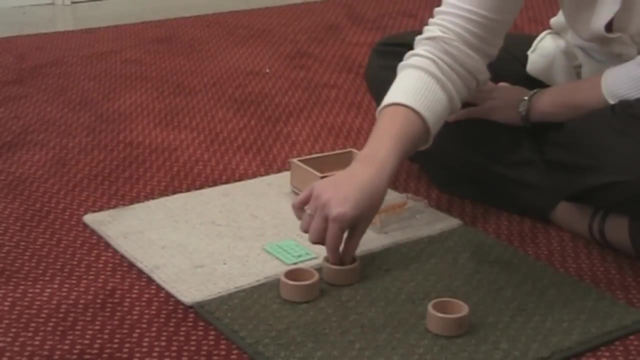 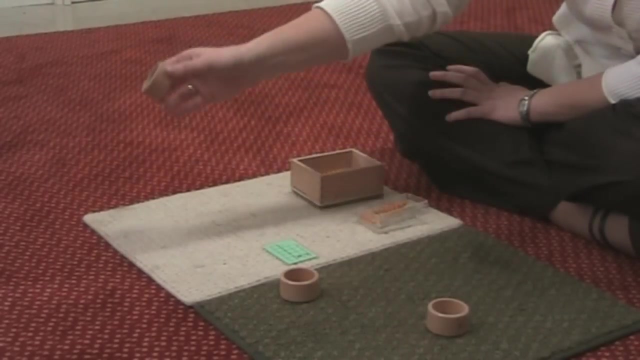 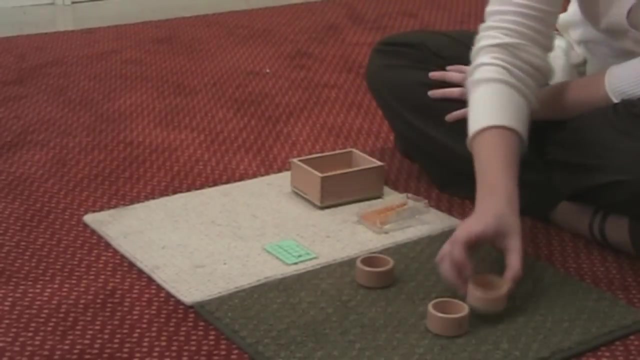 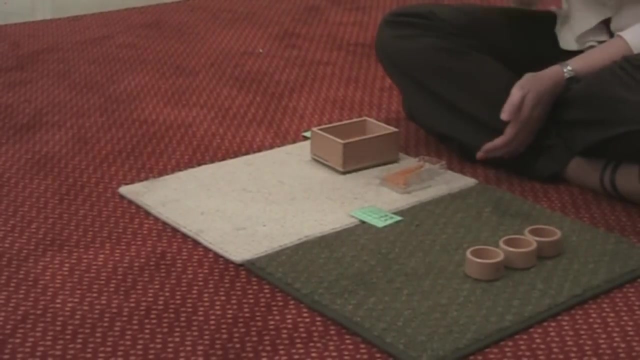 In my next cup I will subtract six beads: One, two, three, four, five, six. How many are left? One bead: Okay, we're going to do a static subtraction with two digit numbers, So we have 58 minus 24.. We're going to start with our units and count eight beads into this cup One. 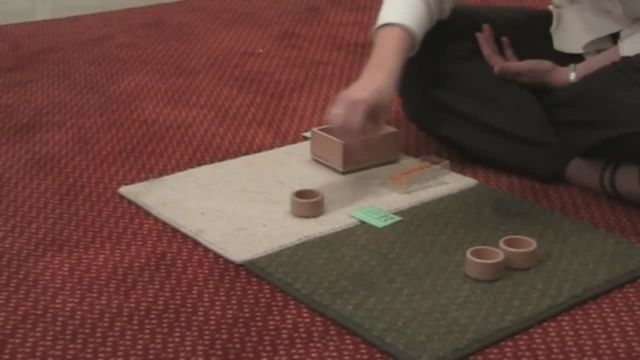 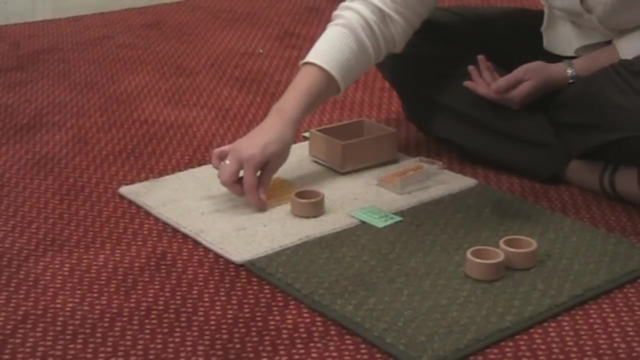 two, three, four, five, six, seven, eight. Now we need to take out five tens to make fifty: 10,, 20,, 30,, 40,, 50,, 58.. word a and 4rgtaWa2tbwfmg. Th3su2, Chinaw. 3gta2wa3gest introduced. 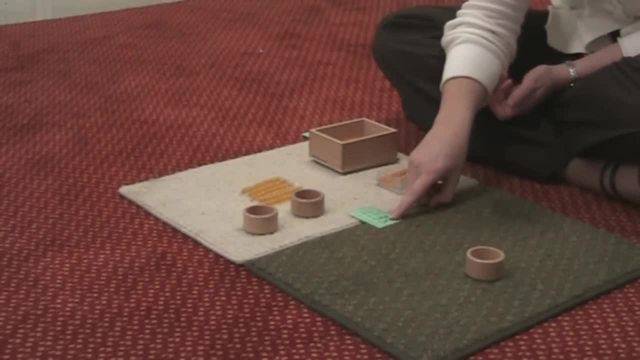 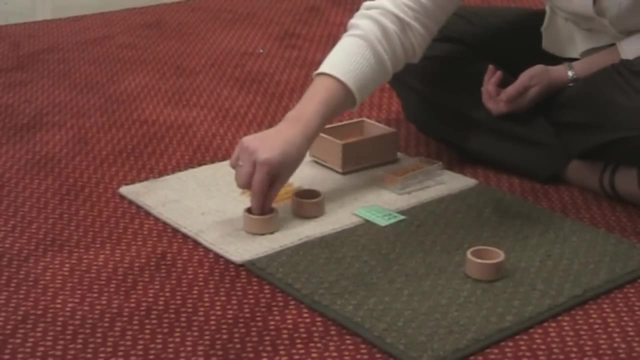 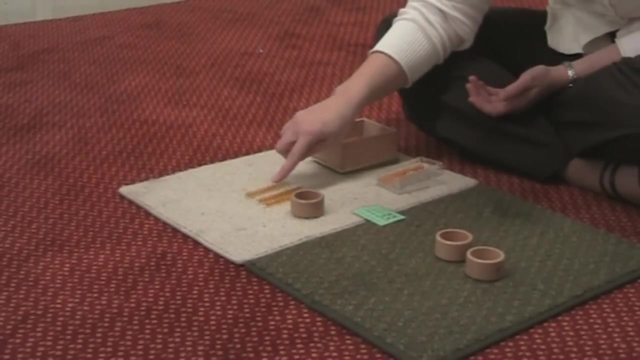 B, where we're going to take away four units: One, two, three, four. Now we need to take away two tens, One, two, and our answer is ten, twenty, thirty, thirty-one, thirty-two, thirty-three. 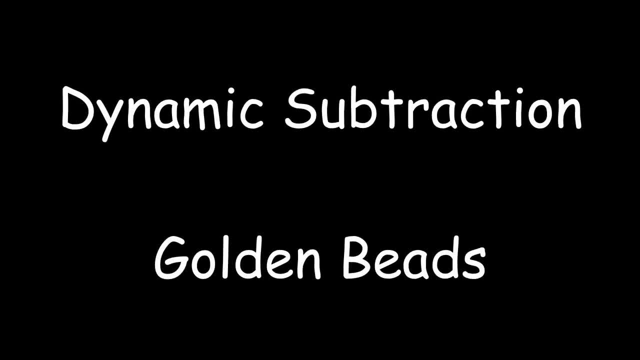 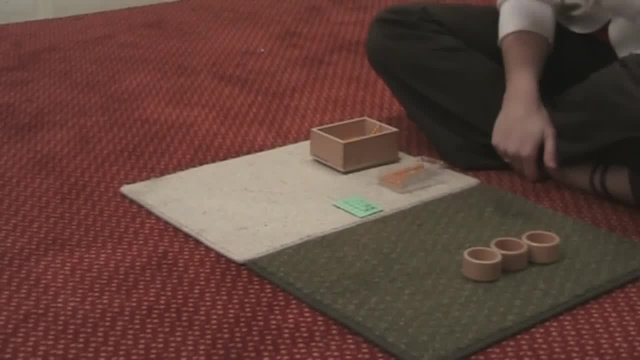 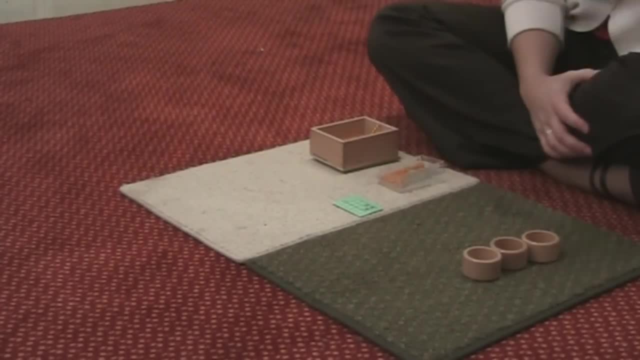 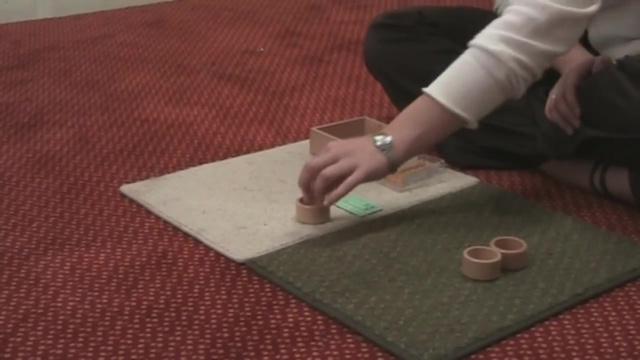 thirty-four. Now we're gonna do dynamic subtraction and I'm gonna show you how we do it two different ways. seven-year-olds use the golden beats, so I'll show you that first, and then we'll use a stamp game second. so we have 26 minus eight. start with our units one, two, three, four, five, six, move to our tens. 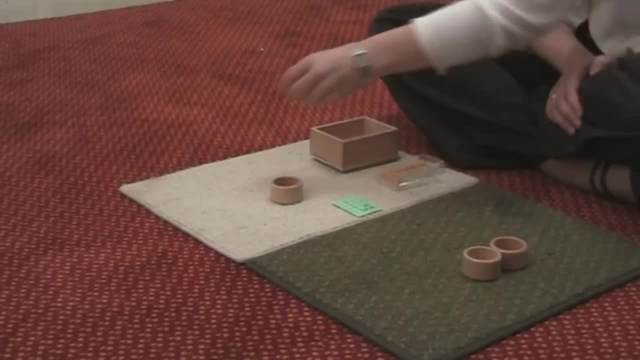 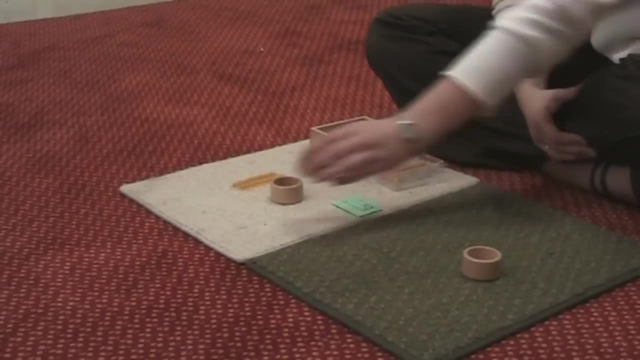 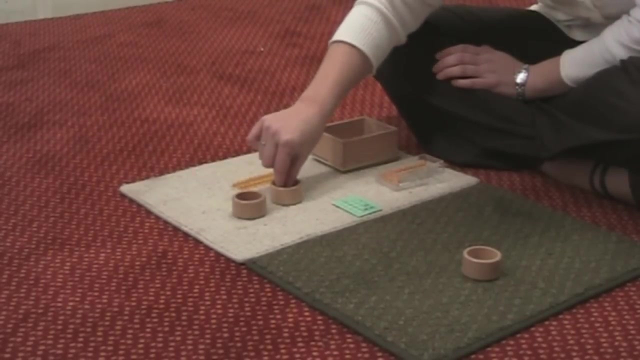 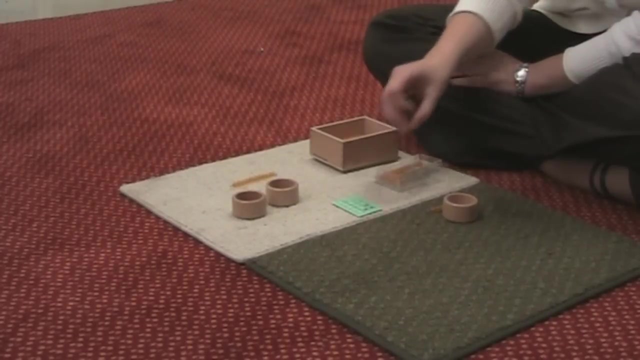 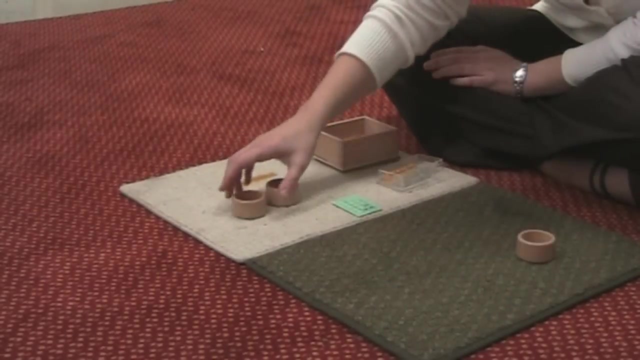 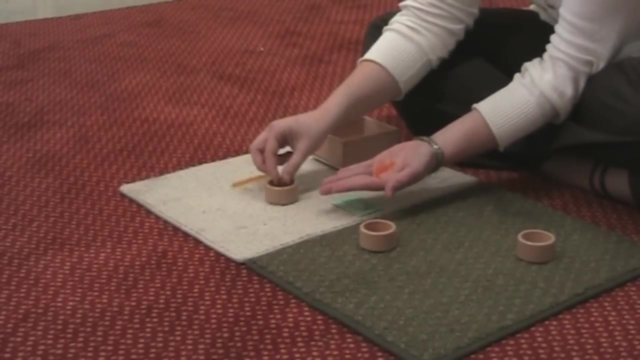 22, 20, 10, 20. now we need to take away eight. one, two, three, four, five, six. uh, oh, I didn't have enough, so I'm gonna take my ten and turn him into ten. now we can take away our eight. see how many we have left. we'll put them in my hand so you guys can see one, two, three, four, five, six, seven, eight and one ten. so we have 18. 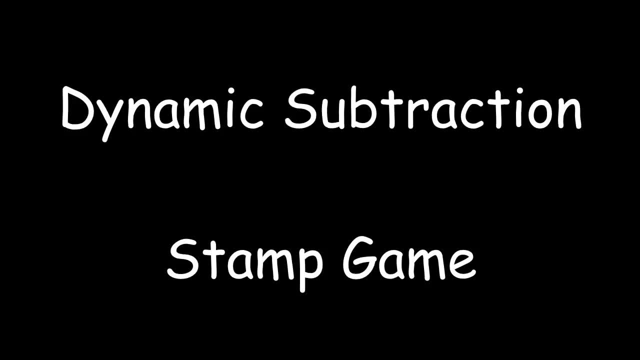 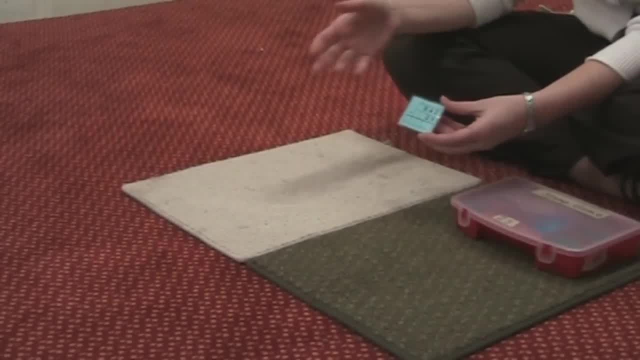 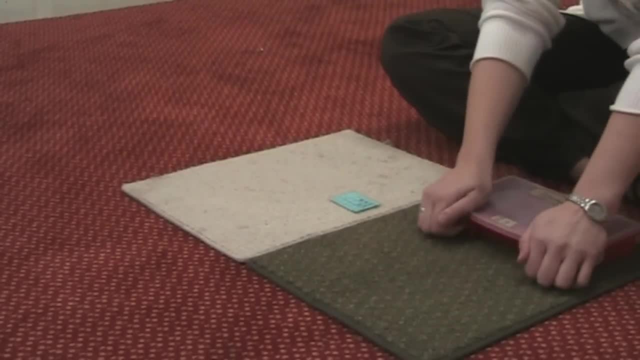 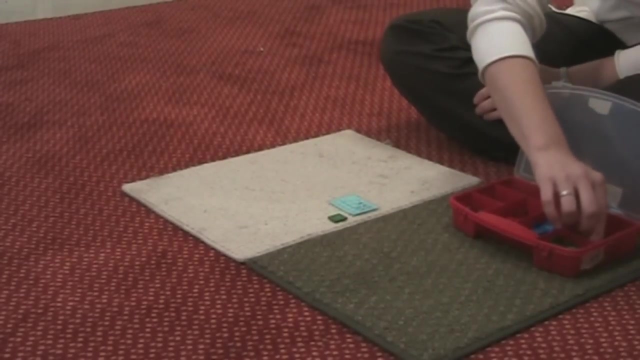 this is a blue card for dynamic subtraction which the older seven-year-olds, eight-year-olds and nine-year-olds would do, and they would do this after they've mastered the golden beats. so we're going to start by setting up our number, always with the units. so we have one, two.